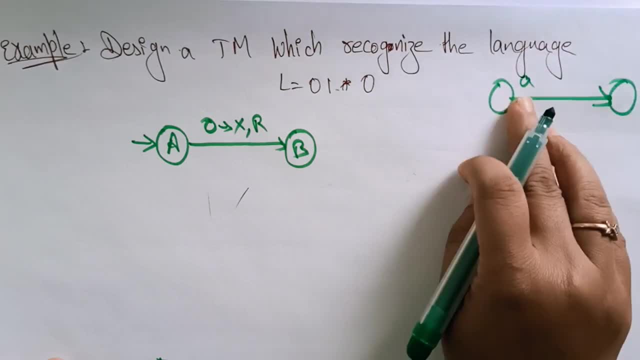 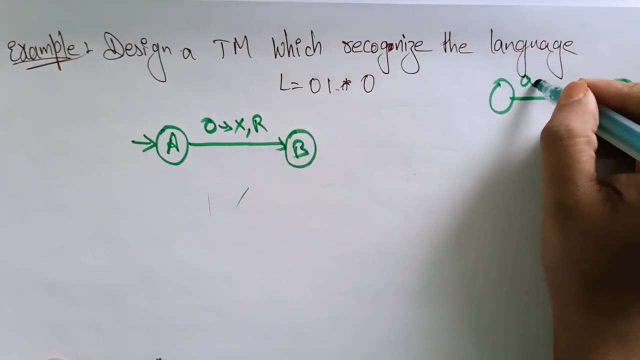 the condition. What is the transition that has to be the symbol to read, that is A. So here, the symbol that is the read that has to be read is 0. Okay. And the symbol that has to write in place of A. whatever the symbol that you are writing, that you. 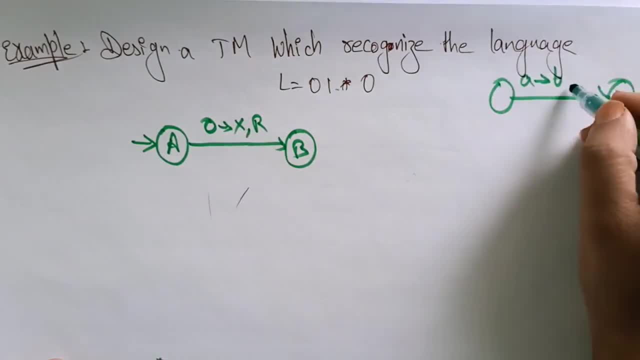 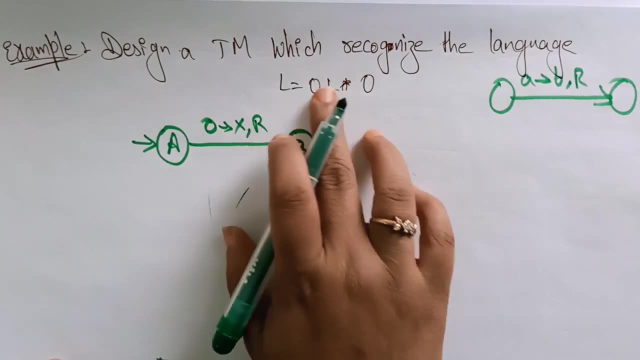 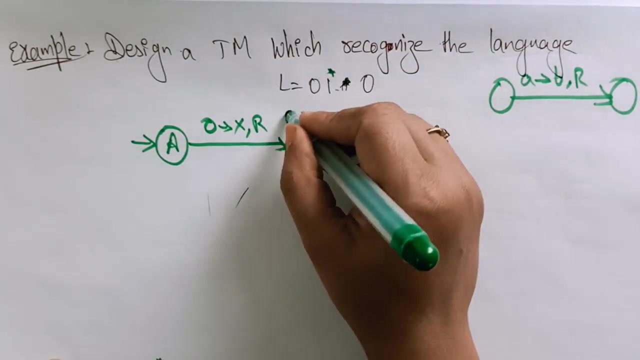 have to write here. The symbol that has to write is is a, B here and it is moving to the right direction. Direction to move either right or left. that you have to mention here. Okay, so 0 is over. Now 1, 1 is multiple. Okay, this is a 1 star. 1 star multiple means you have to take like this: 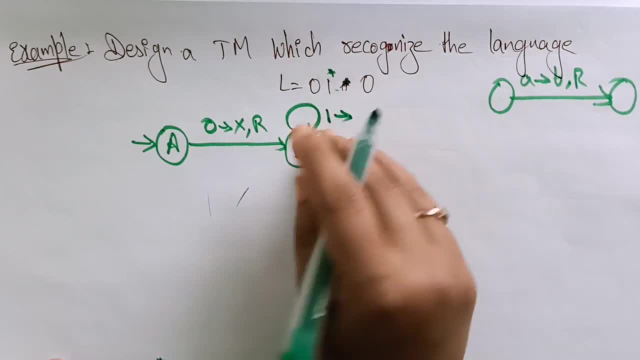 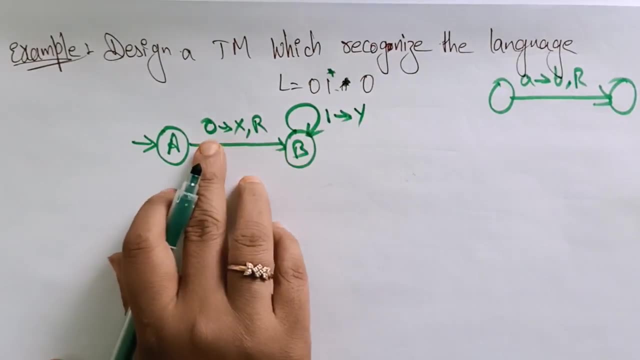 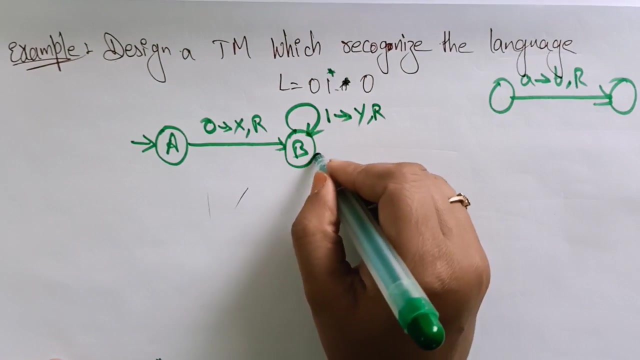 the 1.. Okay, 1, 1 should be 1, 1. I have written, Read and that 1 has to be right as Y. So 0 has written as X with a new variable and 1 has written as a Y and it has to move to the right direction. So again it is going to another state because 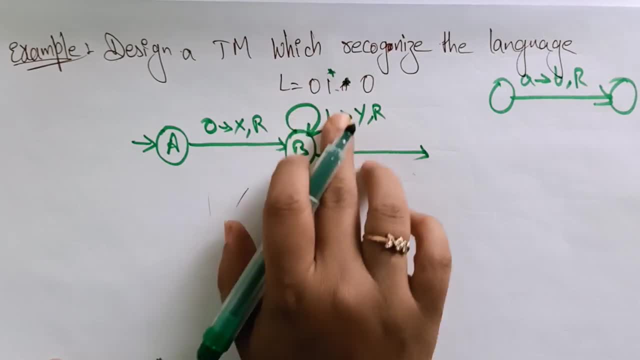 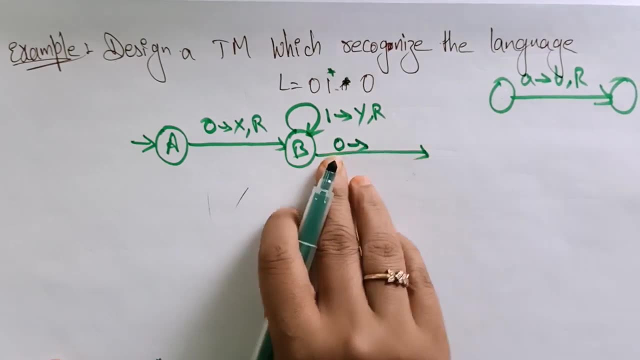 after 1, so it is multiple. 1 star means it is rotating like. this means based on how many number of ones that we are using. Next is a 0. So 0 is read. You are reading the input, 0 and 0 is replaced. 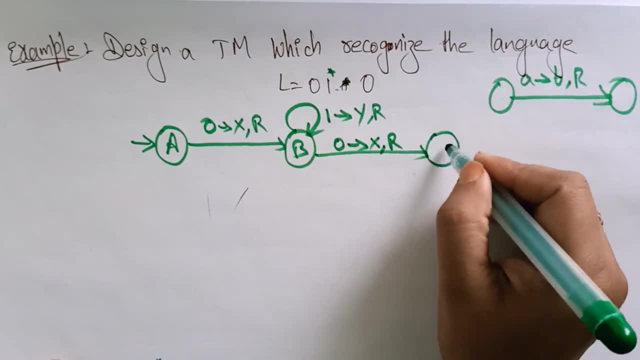 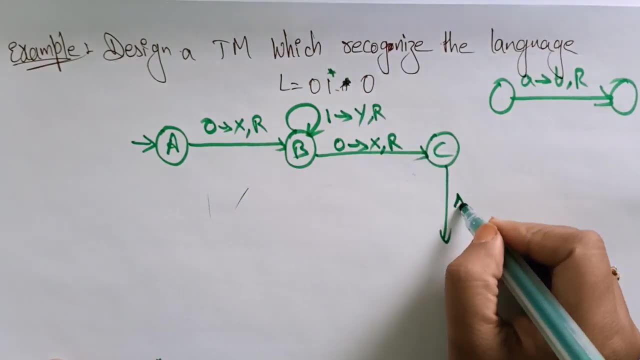 with a blank, So 0 is read. You are reading the input 0 and 0 is replaced with a blank. Now C, so after 0. anything is there, Nothing is there, So that is an empty. It is a blank. 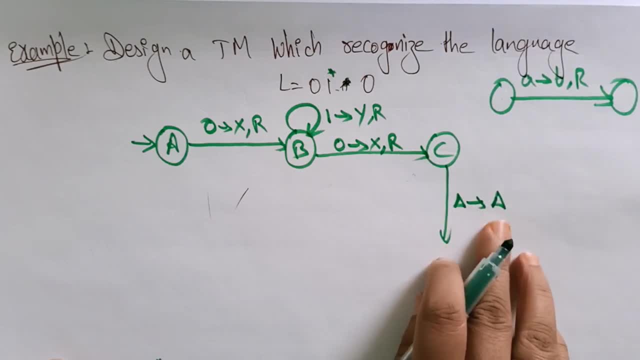 So blank is replaced with the blank. only The blank is replaced with the blank and it is moving to the right direction. So whenever I reach the blank, it is accepted. Okay, suppose if I take the string example is 0, 1, 1, 1, 1, 0 like this: So 0 is read, You are reading the input 0 and 0 is replaced. 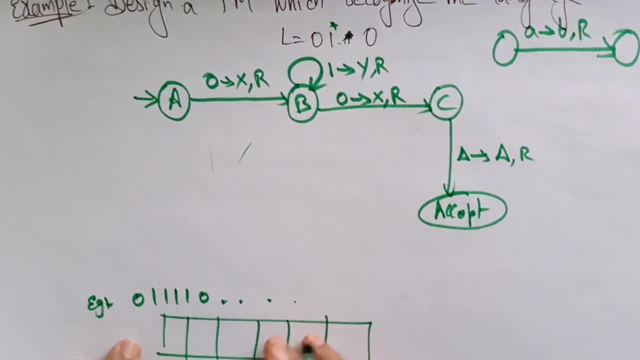 like this: If I take it means 1, star means I can take any number of ones. So 0 I placed Okay, and 1, 1,, 1,, 1, 0, and here it is a delta, is there Okay? so first 0 I replace with X and move to the 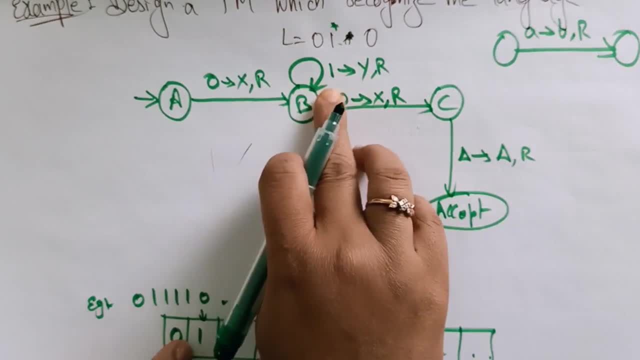 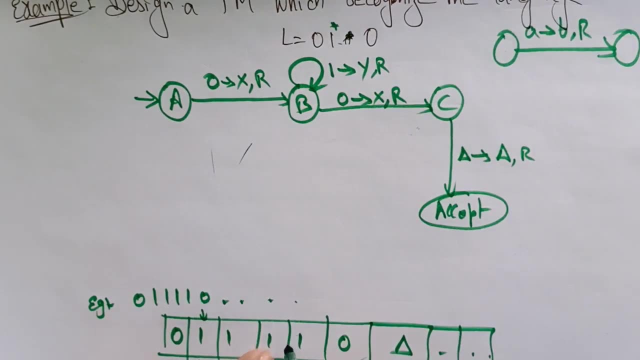 right direction. and again, the 1,. the 1 has to be replaced with a Y. Again, 1, 1 has to replace with a Y. Again, 1, 1 has replaced with a Y. The head is moving towards like this: 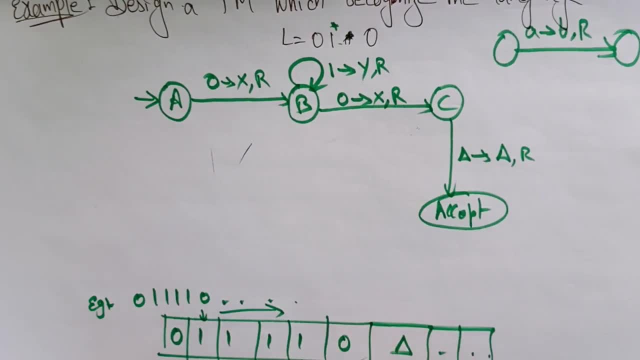 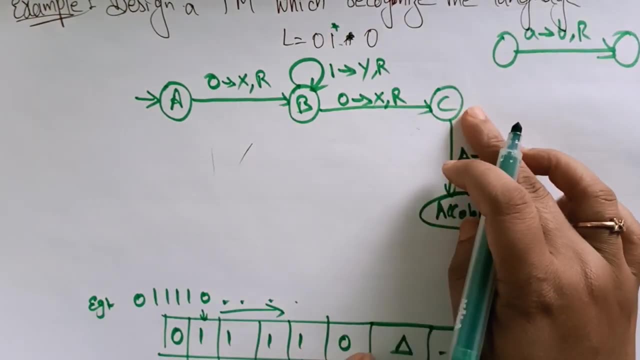 Towards right, every time right. So again the 1 has replaced with the right. So next time, this time 0 has come Means I read the 0. So 0 is replaced with the X. and moving to the right, Now the head become come here, So it the blank is replaced with the blank, only The string is. 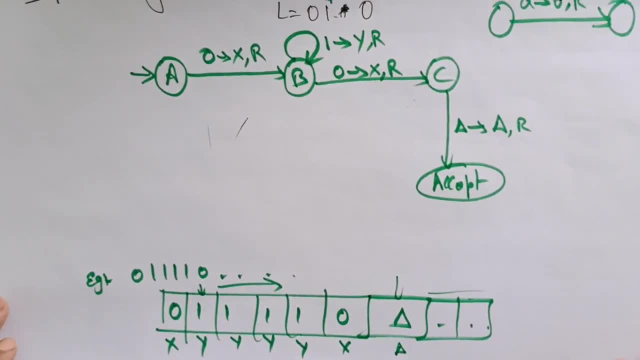 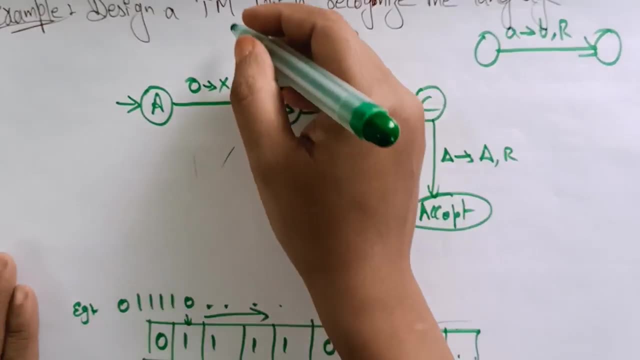 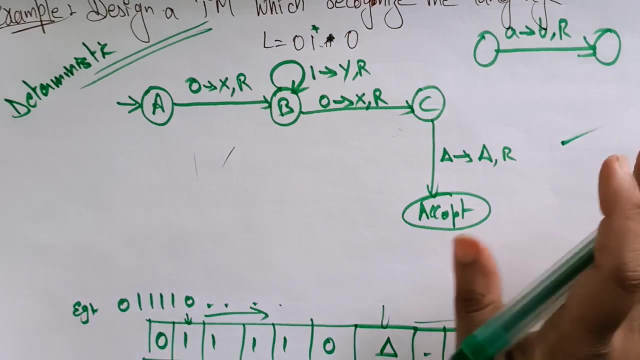 accepted. So in this way you have to be right. So, but here the designing a Turing machine, This is only for the string I have taken. So I said the Turing machine is a deterministic Turing machine. Deterministic Deterministic means actually: this is the correct, If you want. 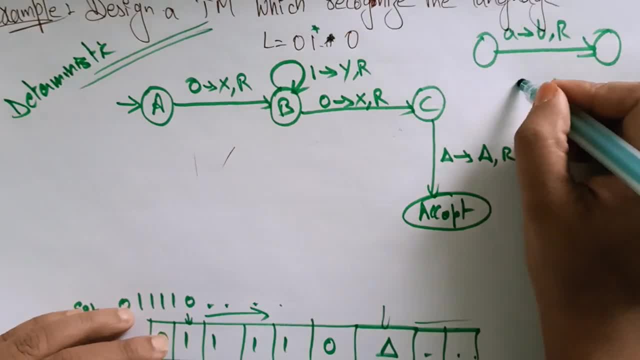 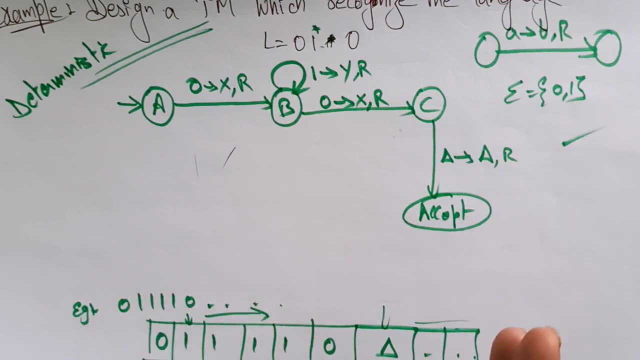 you can take 0 as well as the 1, because the input alphabet is 0 and 1.. So whenever you write the transition, the state is moving from one state to another state. If it is, the input is 0. in the same way, you have to take the input 1 also. Okay, so for input 1.. Okay, for input 1, I am replacing: 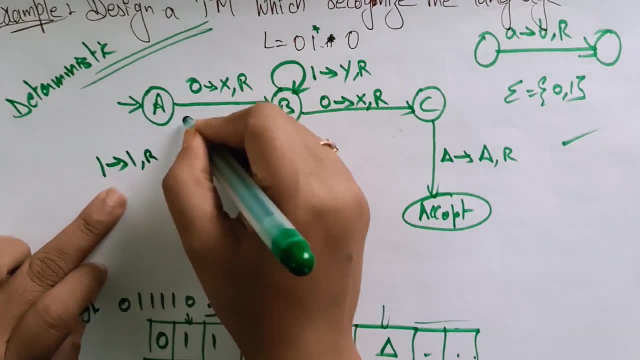 with 1.. So for input 1, I am replacing with 1.. So for input 1, I am replacing with 1.. So for input 1, I am replacing with 1.. Okay, and it is moving to the right direction. It should be rejected. 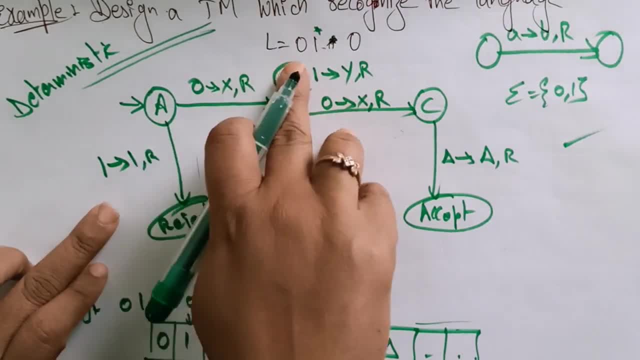 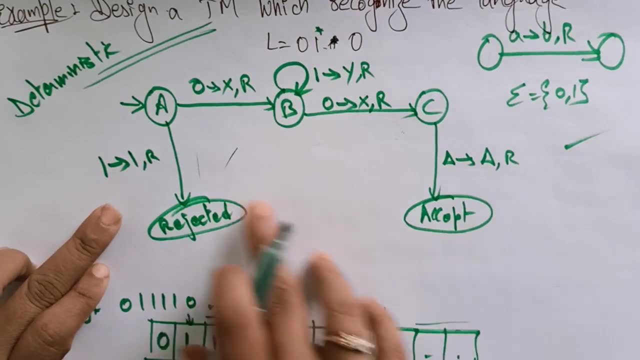 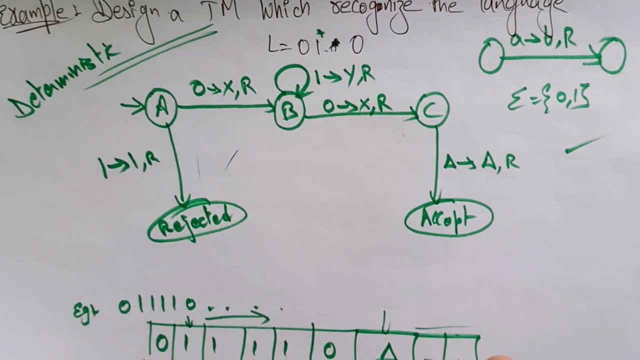 Only this 0 has to be accepted. This 0 because a while going to 0, it has to replace with X and moving right. next one. This has to be this way is accepted, and the remaining all the ways are rejected. Okay, so if you write the rejected and if you didn't write, no matter, that is okay. 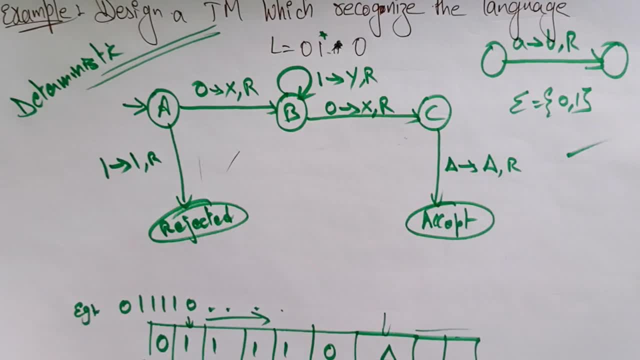 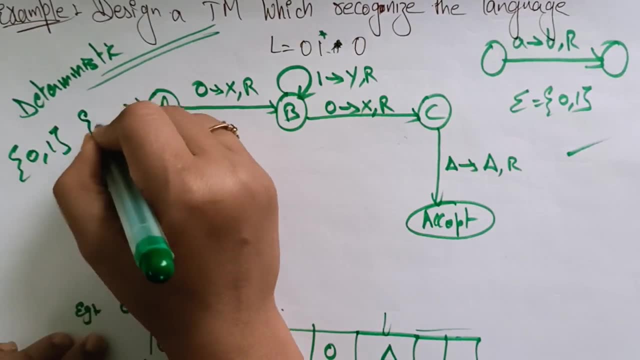 but the accepted way should be: flow should be written. So in the same way, if suppose not only the input alphabets here should be the 0 and 1 and some blank spaces also be written. So 0 is written and the 1 is written and the blank space is also. you have. 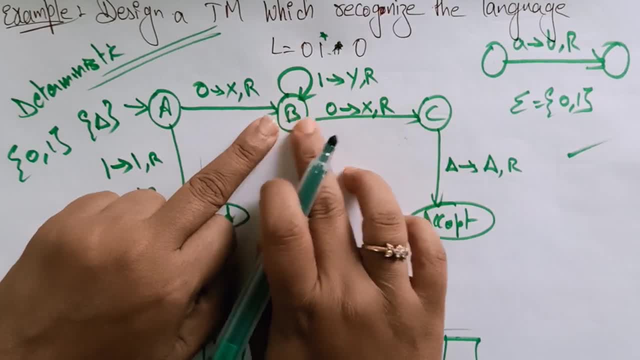 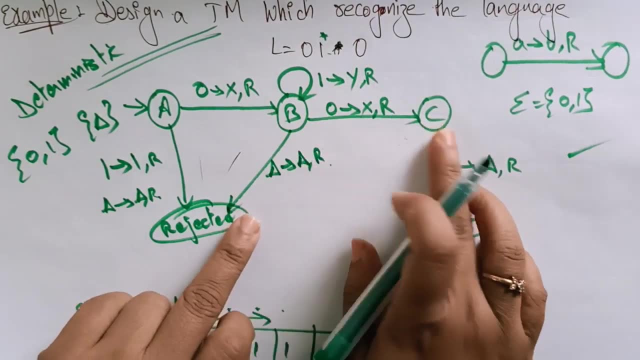 to be written. So here for B: 1 is already there, 0 is already there. So write for the blank space: blank is replaced with the blanks. and moving to the right Now, see, see, blank is there. 0 and 1 is not there. for 0 and 1, it should be rejected. 0 is. 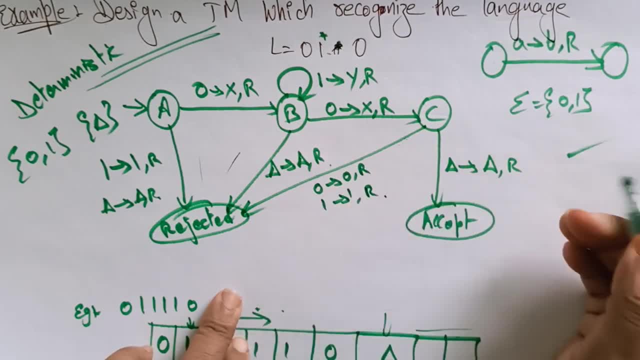 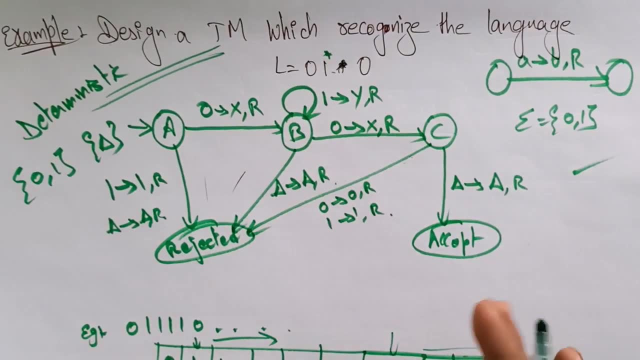 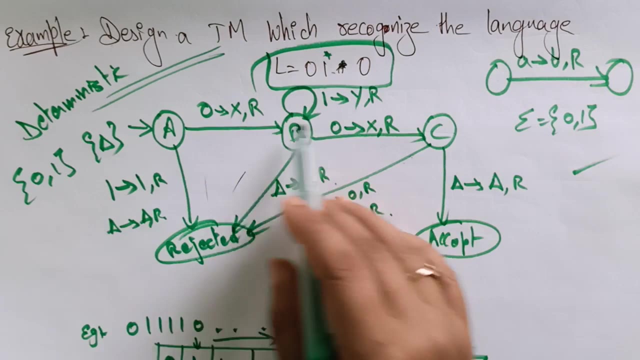 replaced with 0, moving right. 1 is replaced with the 1 and moving right. Okay, and this is the thing. This is the final accepted. See, this is how you need to design the Turing machine. So designing Turing machine for the given language. So first construct, take the input variables and